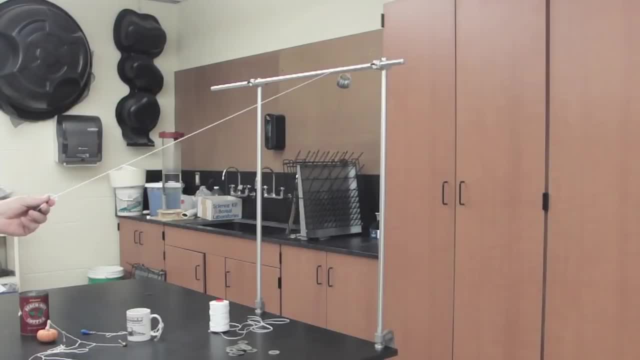 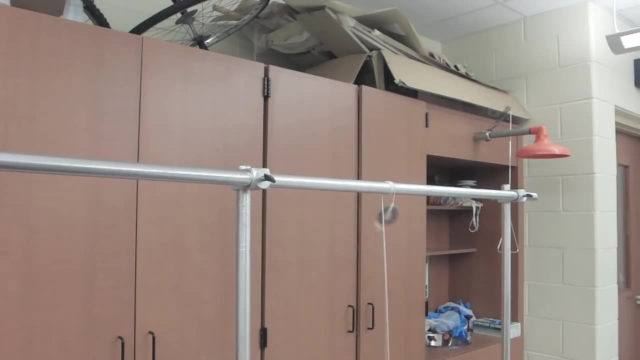 ratio of about 14 to 1.. Other variables to investigate would be the ideal angle to release it from and also what is the ideal string length. Now let's see if we can get a better view of just what's going on in this demonstration. I've added a green LED light to the light. 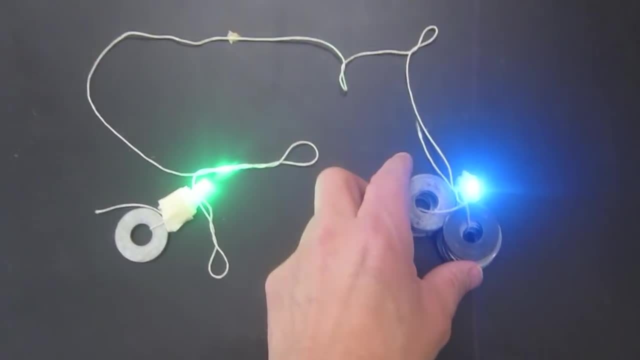 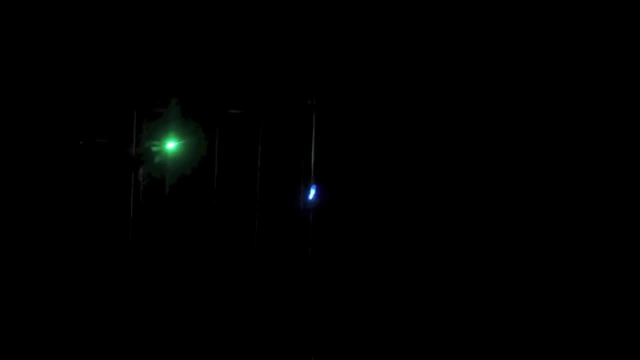 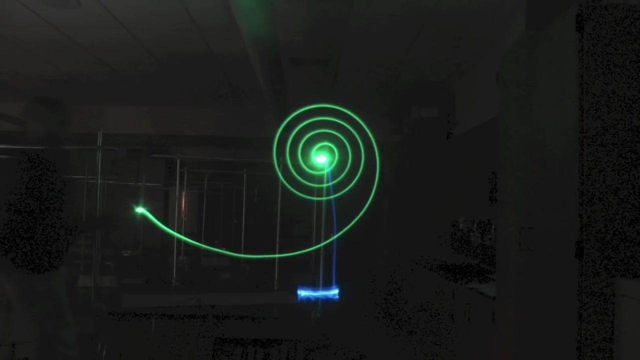 weight and a blue LED light to the heavy weight, and then I'm going to record them in the dark and see what kind of results we get. Now let's try it in the dark. We can see the initial movement of the single weight is to swing down like a pendulum. but 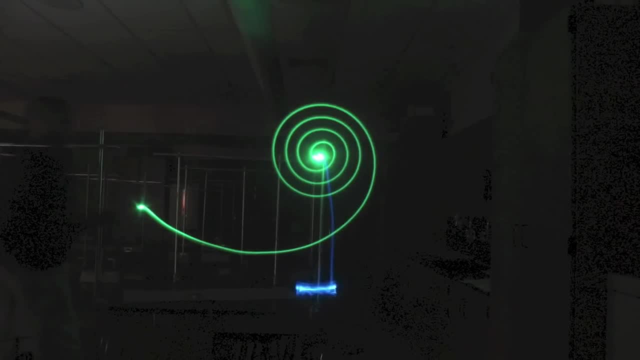 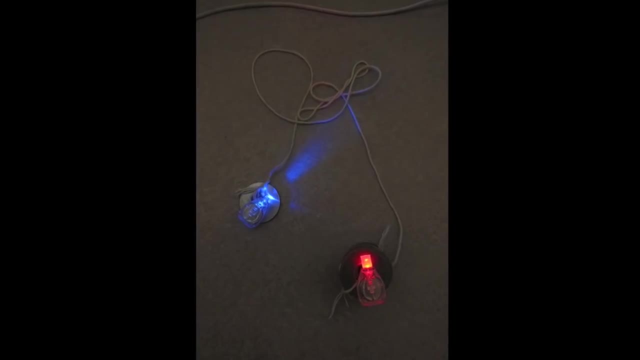 the heavier weight forces it upwards, causing it to loop around. the support Friction stops the heavy weight from falling when that little weight is about the same height as the bar is. Now let's try it again with different colors. Once again, we see the same result. 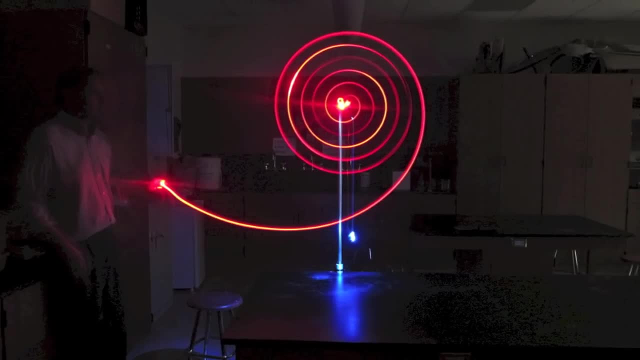 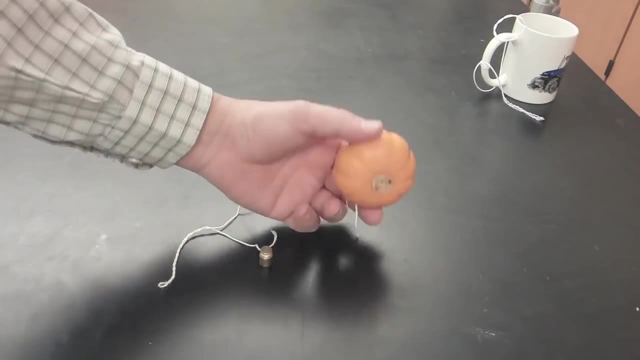 As that weight wraps around the bar, the width of the path stays the same until it reaches the center. This is called an Archimedes spiral. Now let's go in and try this experiment with some other materials. Here's a small pumpkin in a tiny weight. Let's see how this one works. 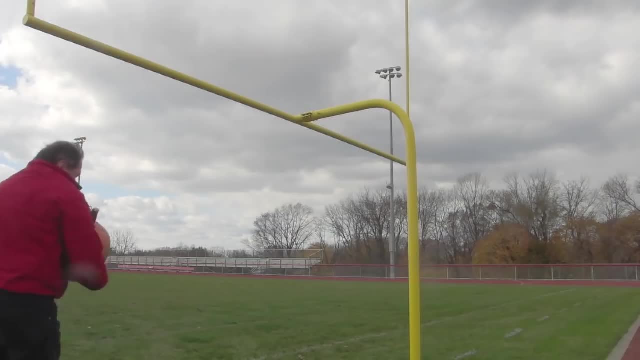 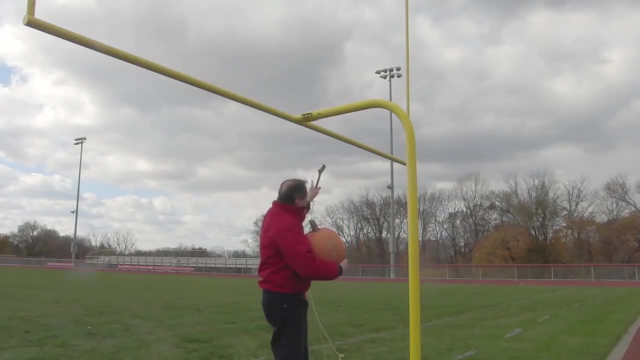 Now let's try it on a larger scale. I have a 21 pound pumpkin, a pound and a half wrench, a 10 foot high goal post and 8 feet of rope. So let's see if it works on this. 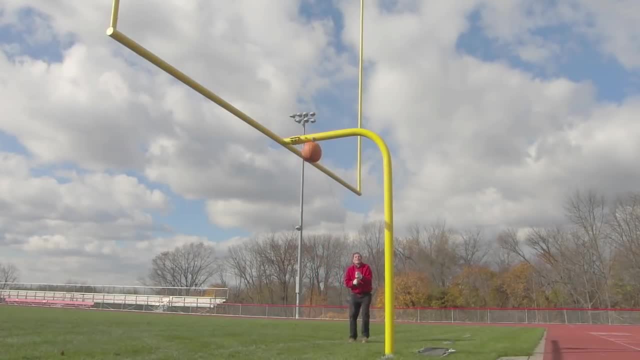 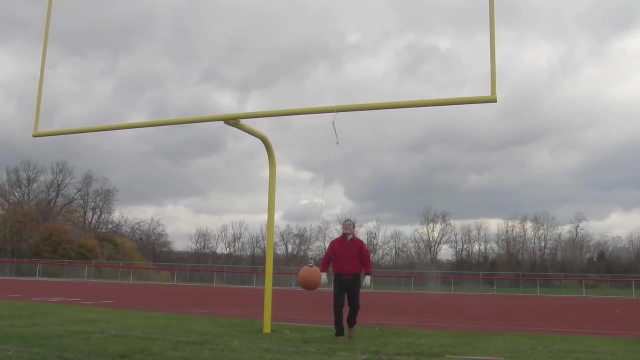 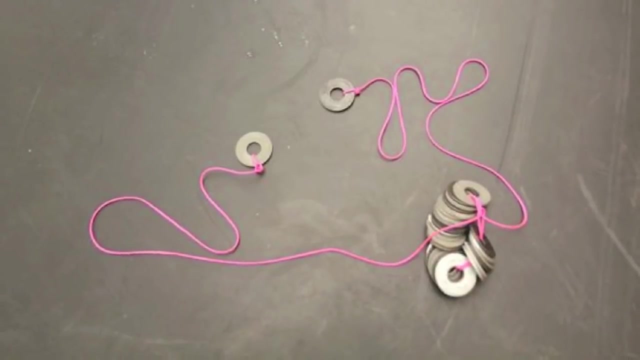 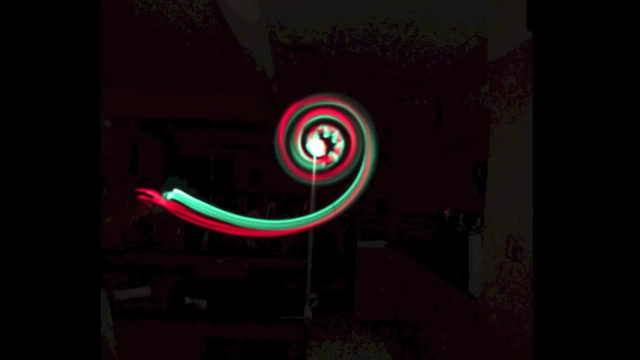 Here's another investigation. we can try Replace that single weight with two smaller weights and two strings. When I pull them out on the same side on release, we see that they both act together as one, as seen by these two coils, And this is the. 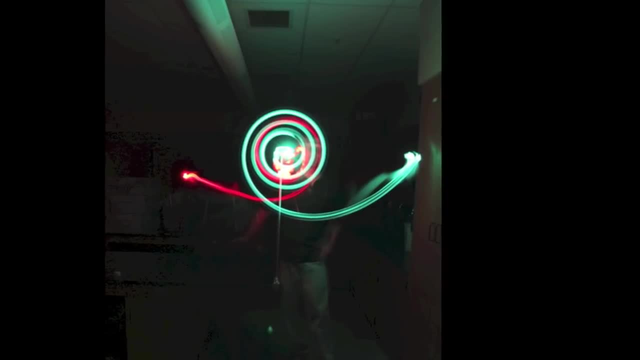 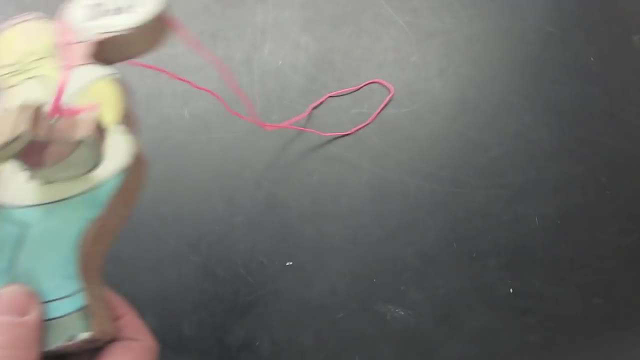 result I get if I release them from the opposite sides of the bar. I also thought this might be fun to make into some type of game. For example, here's Homer Simpson and an axe. Obviously, the point of this would be to have Homer saved by the axe.